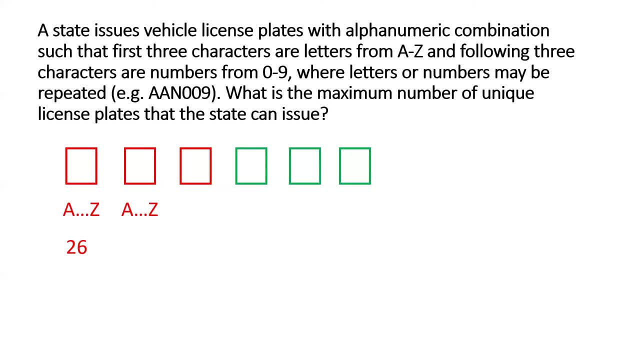 So if we have used, you know, any one letter in the first placeholder that can be potentially used, The same letter can be potentially used in the second placeholder as well. So that's the second placeholder. That's why all the letters from A to Z are still under consideration for the second placeholder. 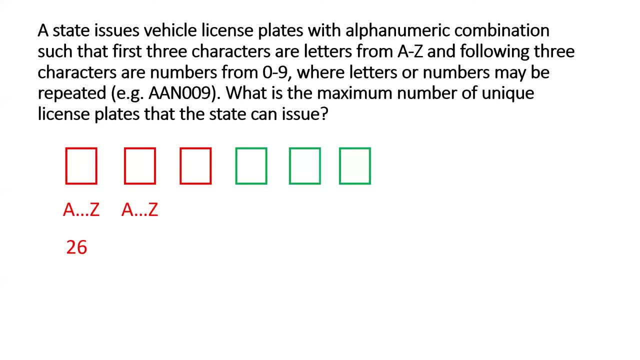 So for each way of filling up the first placeholder, we can fill up the second placeholder in 26 ways. So the number of ways we can fill up the first two spots is 26 multiplied by 26.. And in the same way for the third placeholder, we have again 26 different. 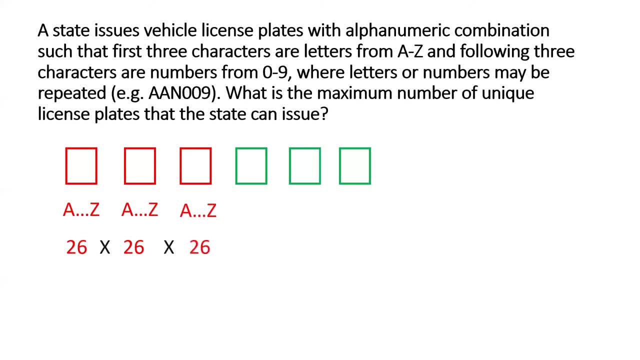 options from A to Z. So the first three placeholders can be filled up in 26 multiplied by 26, multiplied by 26 different ways. So that's 26 cubed different ways. Now let's come to the green placeholder. So that has to be filled by any one of the numbers. 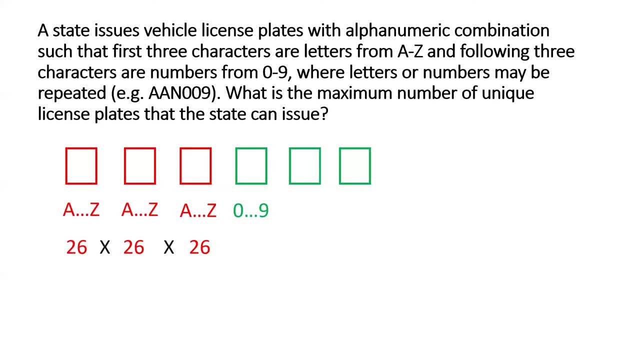 from zero to nine, So it can be potentially filled in 10 different ways. So the number of ways in which the first four placeholders can be filled is 26, multiplied by 26, multiplied by 26, multiplied by 10.. Now for the second green placeholder that also has to be filled by a number And once. 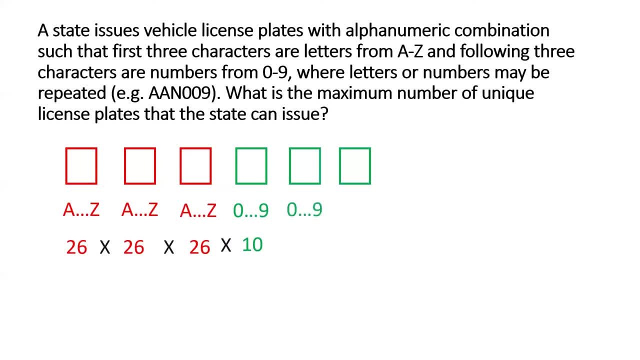 again, since repetition of numbers are allowed, we can consider any one number, from zero to nine. Do you see that this expression is another example of a green placeholder can fill in 10 different ways. So if I see this green placeholder is charity, the green placeholder is charity. it means 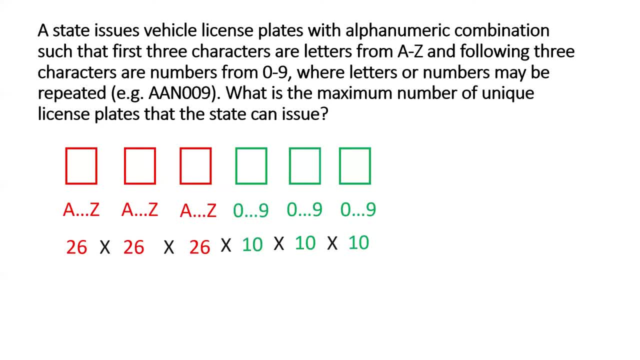 to himself or her, even if he or she is a charity. Something else is important here. It is important to keep looking for things to confirm differences in what we have in the first placeholder. Or another way is to look for something to talk about later. 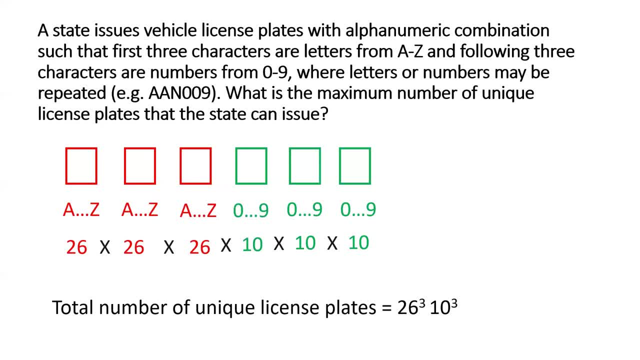 So let'szą it with all pluses. So z's also can be used here. Let's try that. So that makes a total of 26 cube multiplied by 10 cube, And it will be good to leave this at that.